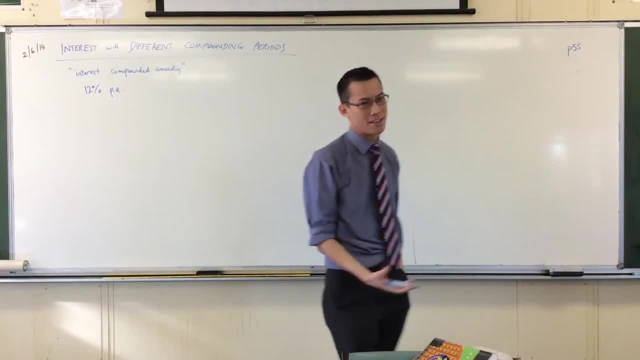 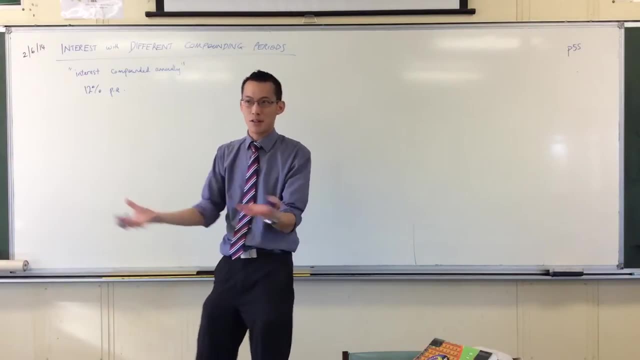 Nice, Not bad right. Maybe there's some stupid high fees or something like that. that makes up for it. Okay, 12% per annum. Now let's start with some sum of money. We generally go with like $1,000.. 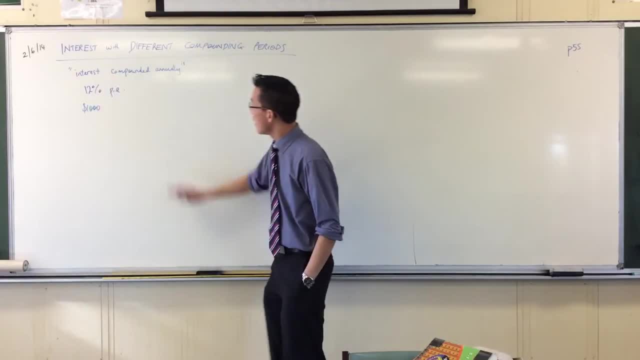 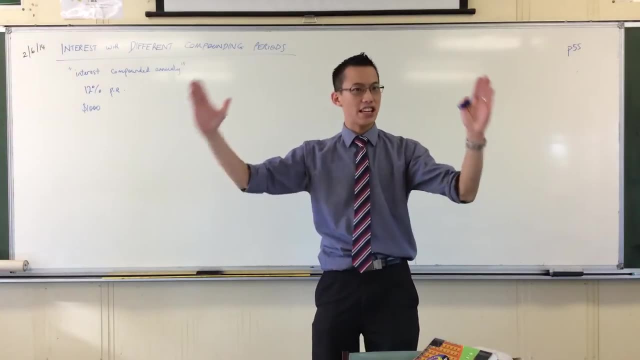 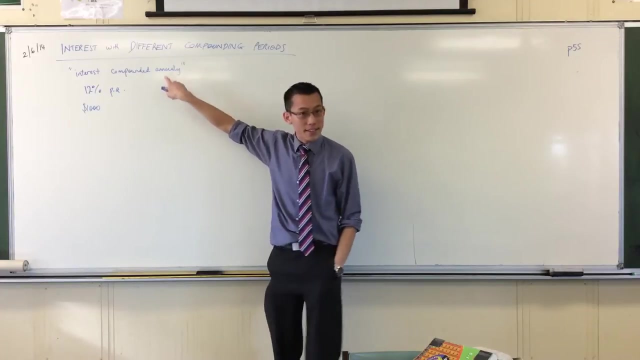 That's a nice easy figure to think about. Okay, now if it's compounded annually, what happens? You stick your money in, right, and for 12 months nothing happens. Your money just sits there, It doesn't grow at all. but then at the end of the year- right, and once a year only- they'll pay you that interest and they'll pay 12%. 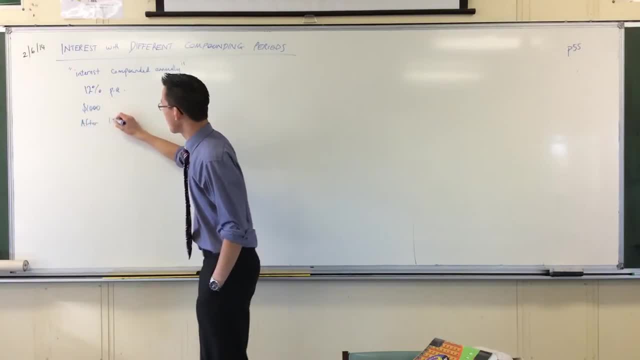 Okay, so it'd be like this After one year? right, you'd have that $1,000 plus the 12% interest, right, So you'd get this: The amount would equal. now, do we remember what the compound interest formula was? 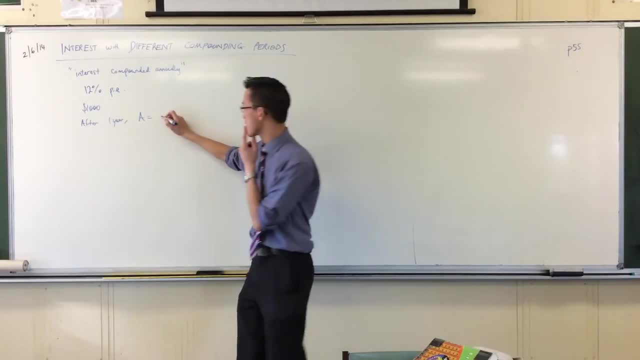 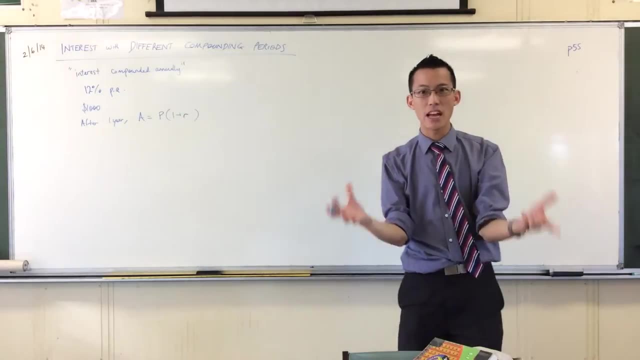 Because that's what this is right. What comes first, P right, the principal times. what's in the brackets, One plus the rate, and then what's the power N which stands for Time, Yeah, time or number of. 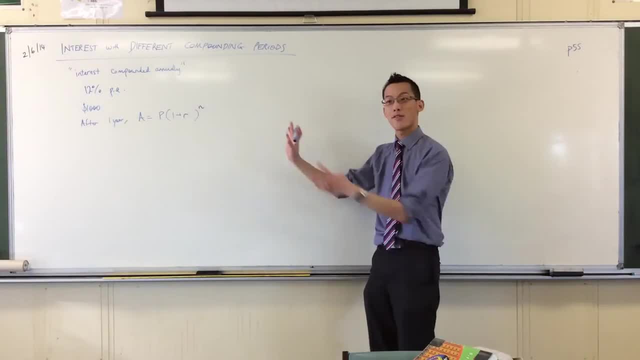 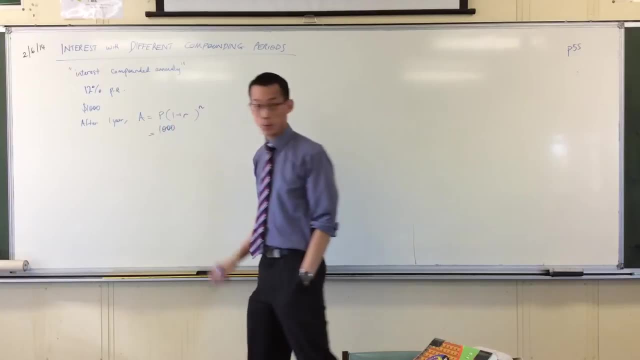 Years. Now, usually we say number of years. okay, Now, that's fine. I don't have my iPhone now, but you'll see in a second that will change. okay, Now let's just calculate the numbers. We said P was the principal, so that's $1,000. 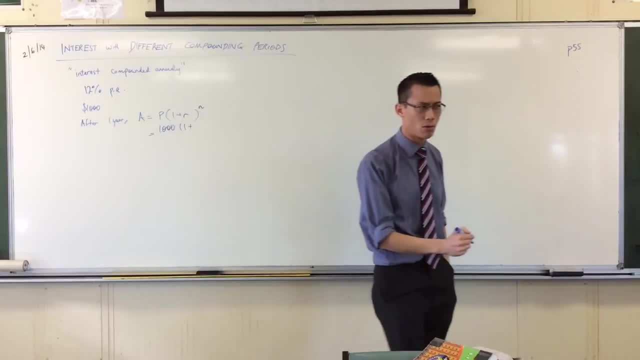 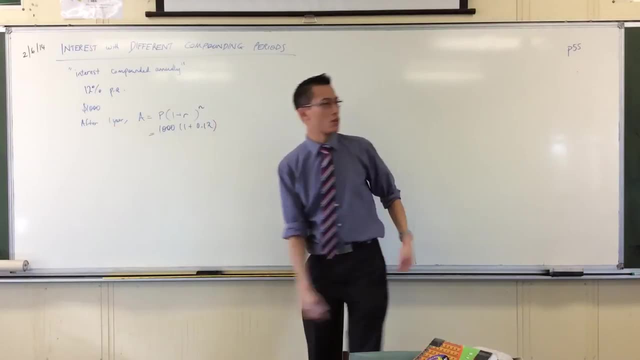 Your rate, 12% as a decimal, What is it? 0.12.. Yeah, 1, 2.. 0.12.. Okay, now it's just in there for one year, so it's just a 1.. 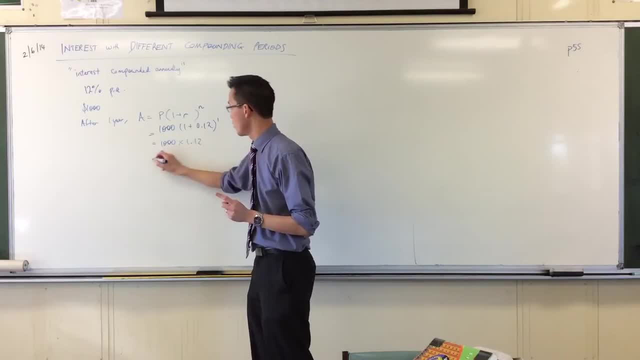 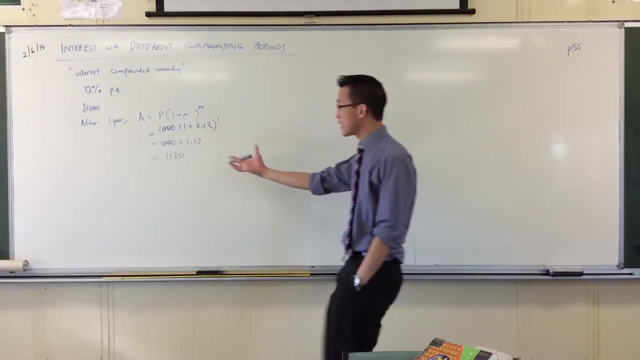 So 1,000 times 1.12.. Last I checked, that's 1,120.. Okay, so that's no big deal, right? If we went for another year, we could go through this whole thing again and we would change. 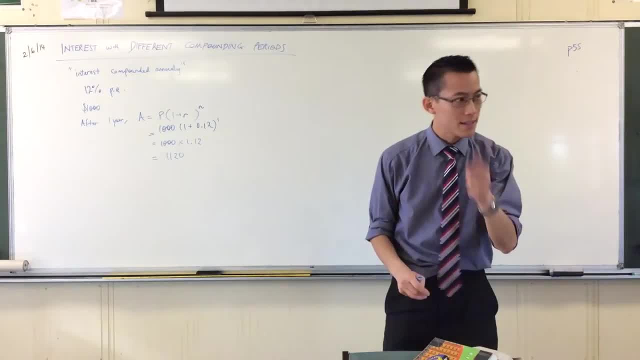 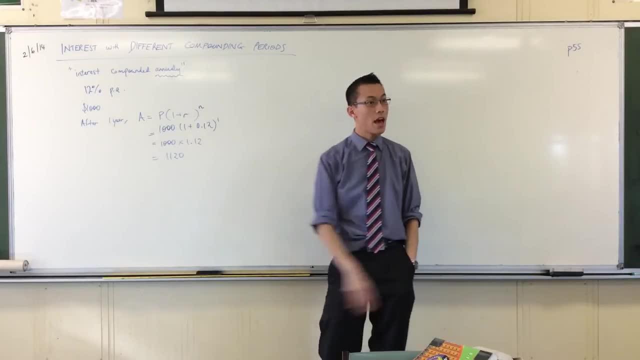 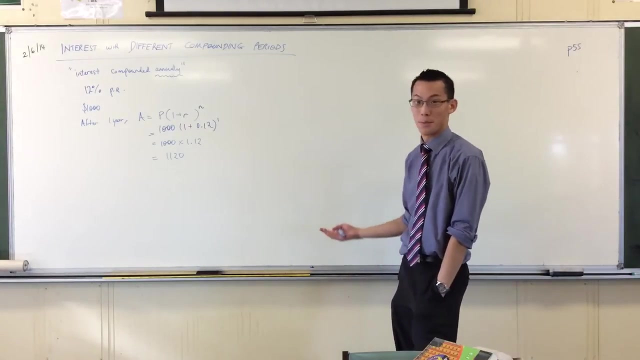 this number up here, the N okay, Ah, but here's the thing: right, Compounding annually. that's a long time to wait to get paid your well, the interest in this case is $120, right, Banks certainly don't wait this long to pay you money. and if a bank did, you probably 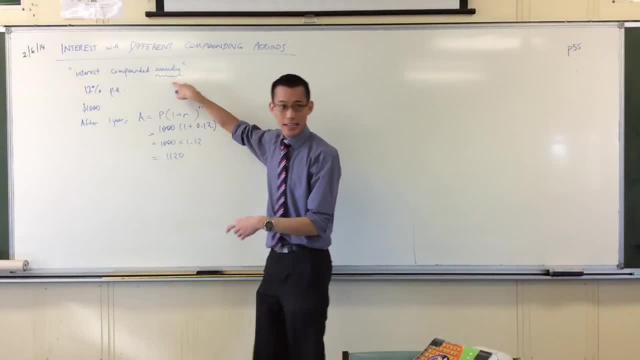 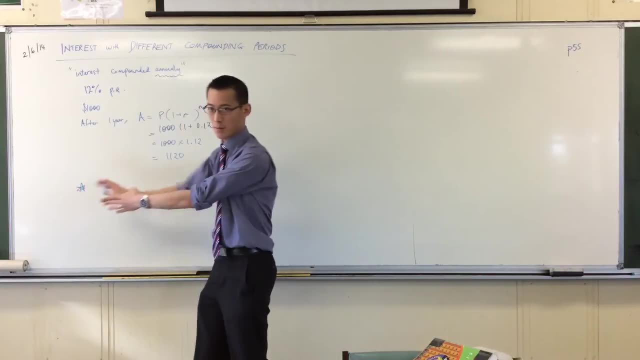 wouldn't go to them, okay. Instead of compounding annually, they will compound annually. They will compound more frequently, okay? So, for instance, you might have: let's do some, let's do some. I'll turn this down here. 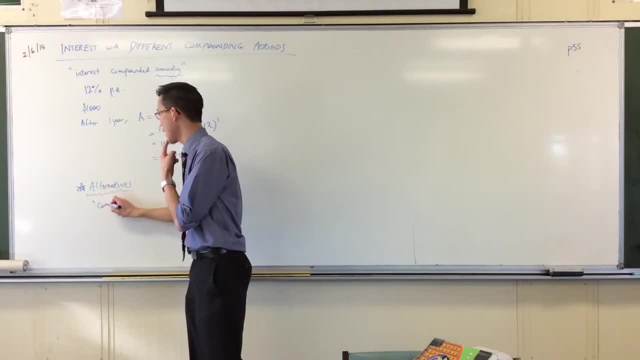 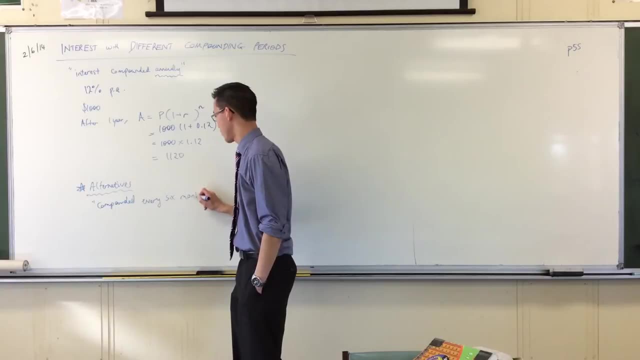 And you'll see questions for all of these. right, You might see compounded every six months. So that means they'll do it twice a year. Okay, now we'll talk about whether it's better or not in a second, but let's just get down. 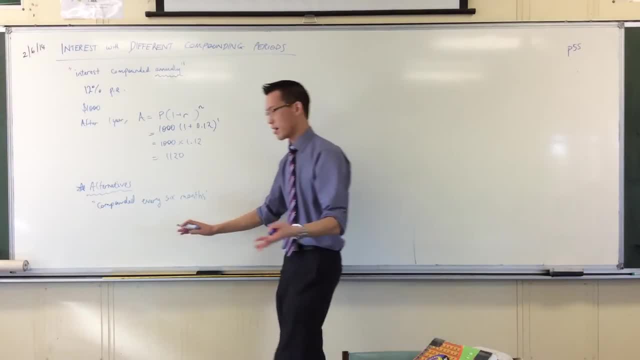 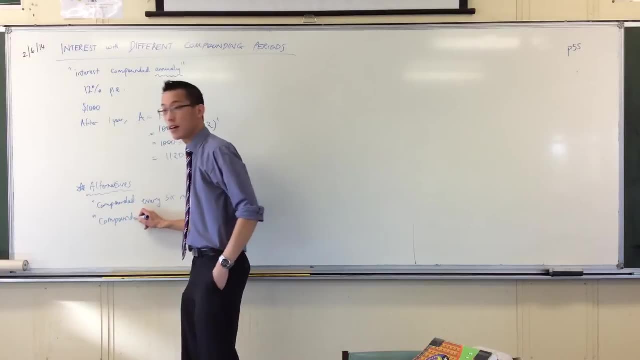 a few different options Compounded every six months. The next most frequent example you come is quarterly right. Compounded quarterly, which is every how many months, That's three months right, Because a quarter of a year is three months. 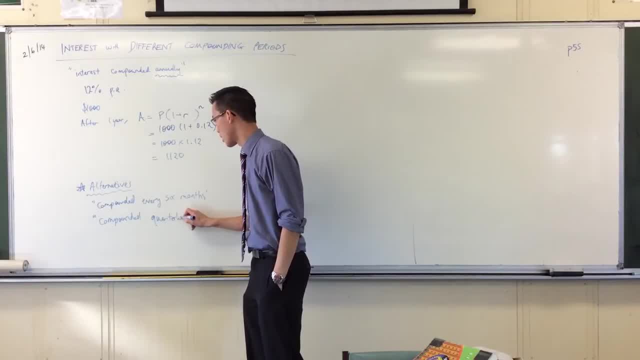 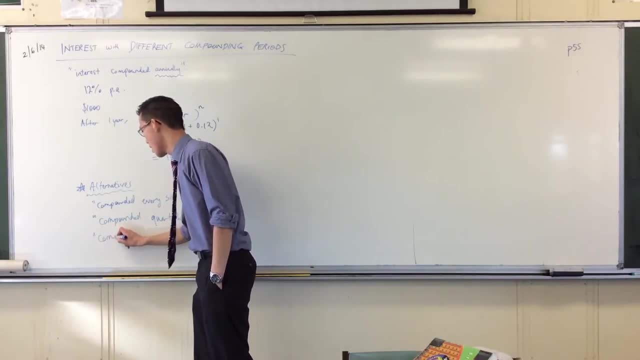 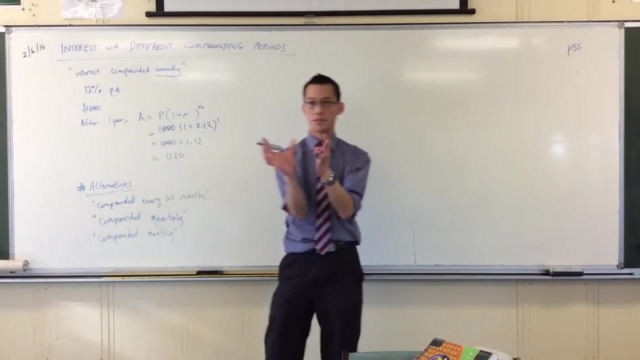 So they might say: compounded quarterly, four times a year, right, I suppose they could compound monthly and you know you could do it, you could do it as any you know any sort of time unit You could do it like, you could do it weekly or you could do it daily, is the most common. 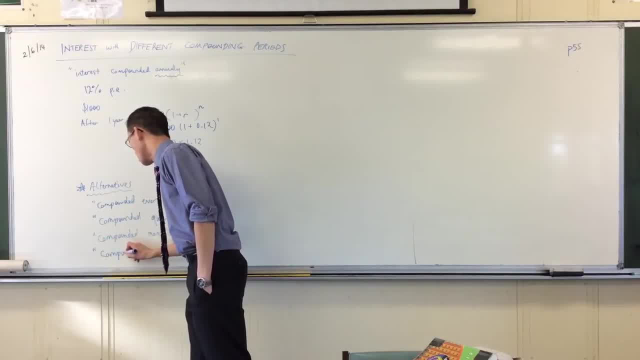 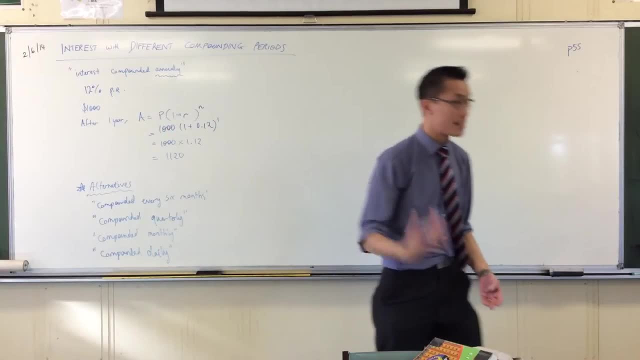 one actually, In fact, your ones, your bank accounts- if you've got one- and I assume most of you do- are compounded daily, Every single day. they're doing this kind of calculation for you, And that's why, when you get paid, you know you only get like four or five cents or something. 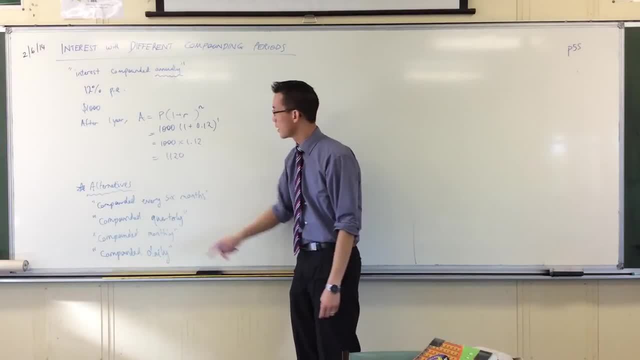 small like that, because it happens many, many times a year. okay, But what happens when we do this, if, if we change the situation? okay, Let's go, Let's go compound every six months. okay, Let's think about our original $1,000 and our 12% per annum. 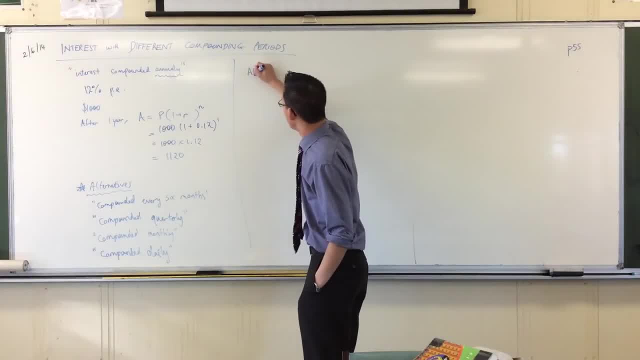 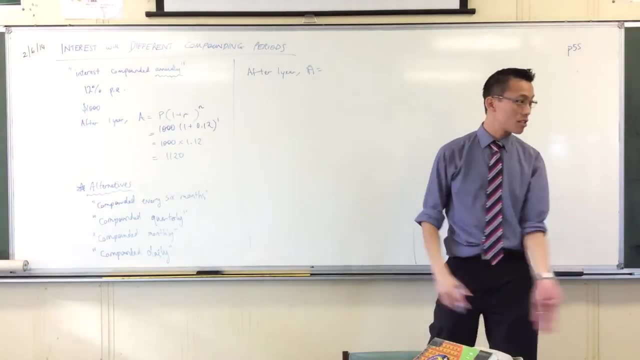 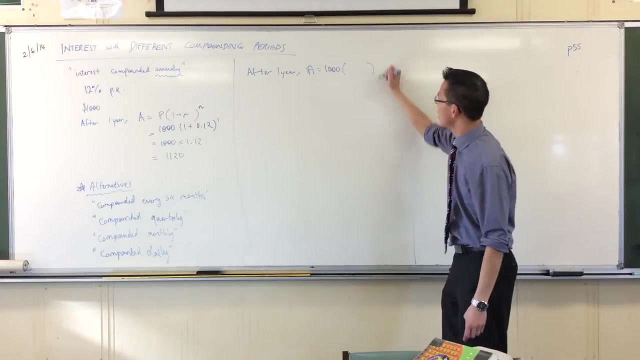 Let's think about this: okay, After one year, what happens? okay, You're going to get an amount right. Your principal is still the same, it's still $1,000,. okay, Now, what's going to happen in here? hmm, I'll leave the brackets for a second. 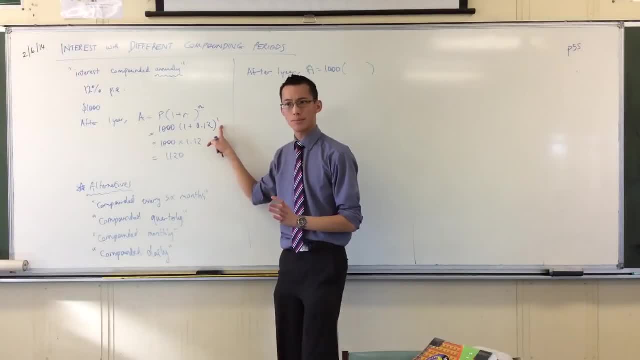 Tell me what would N be. It's not going to be one anymore, Right? It's actually going to be two. Why is it two If you go every six months? right? they're compounding. every six months they're recalculating. 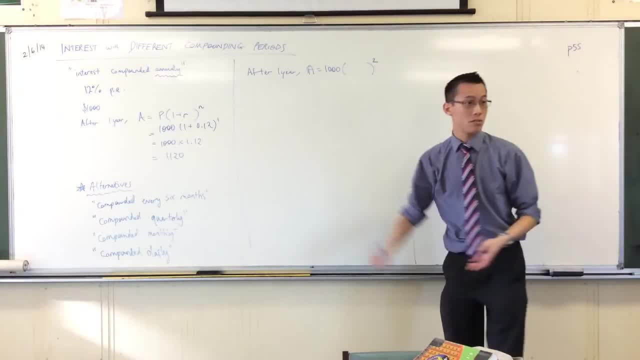 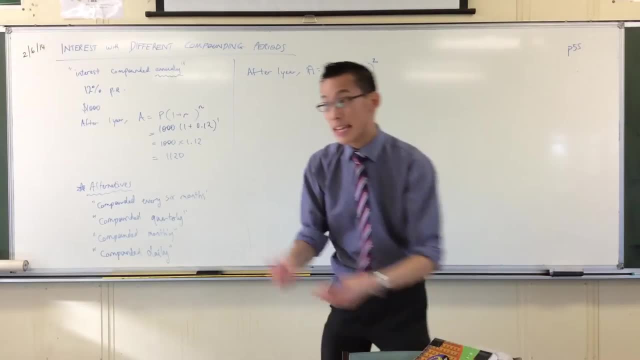 how much interest you get right. So this number up here should be a two, right. So it's not just number of years. Actually, a better way of saying it is it's the yeah, that's right. well, it's two lots. 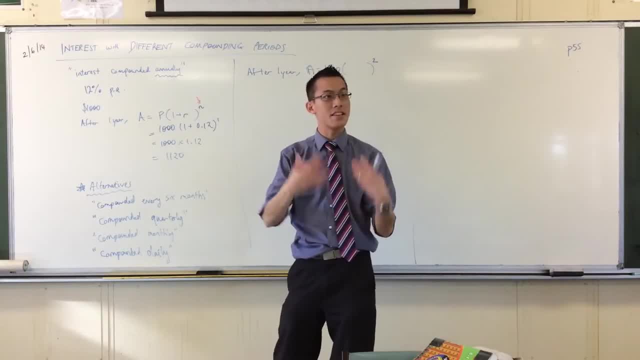 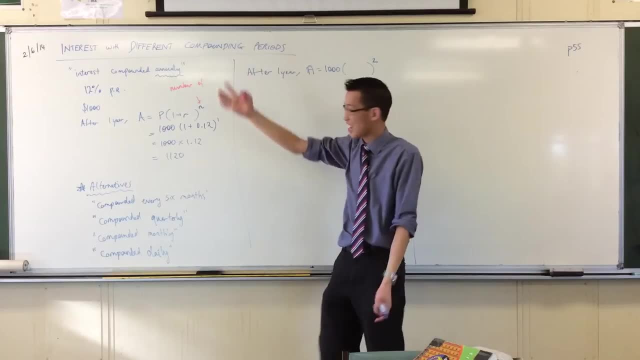 of six months, or a more general way to say it is: it's the number of um compounding periods. Okay, That's this what this thing is actually called, Um. this is a compounding period of a year, or a compounding period of six months, or 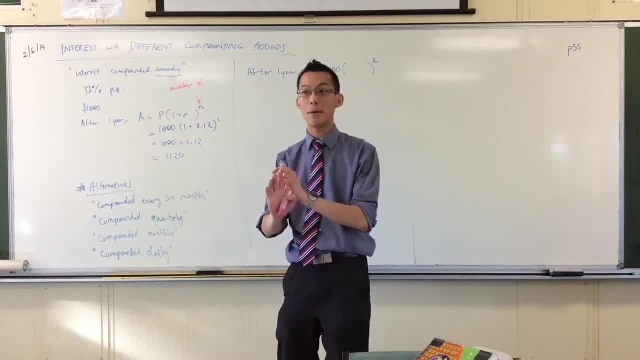 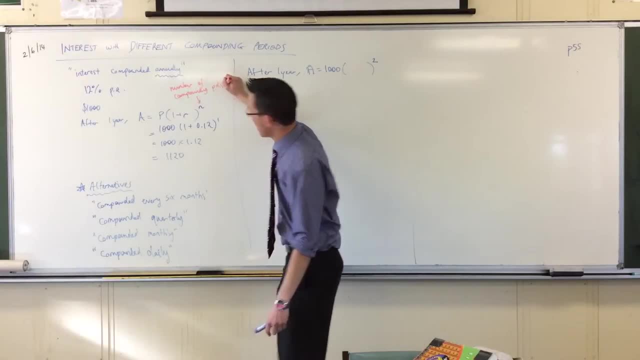 three months or one month or one day. okay, The compounding period can be anything you like, okay, So this is the number of compounding periods and admittedly, it usually is years, but it can be anything we like, okay. 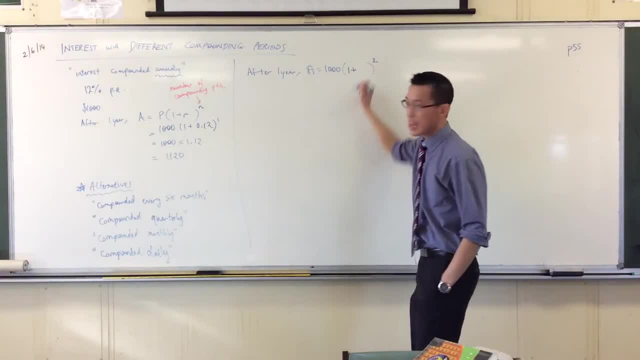 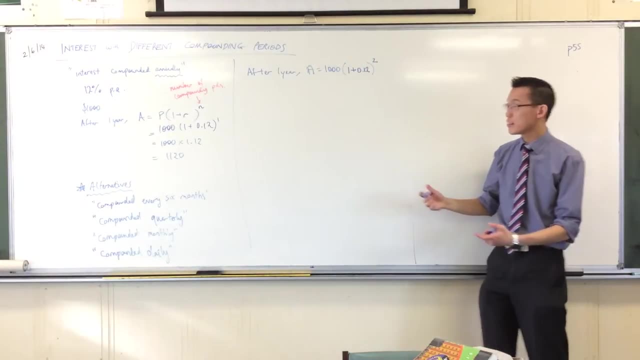 Now a bit of that's been changed to a two. What would happen if I wrote down what I wrote before? Okay, 0.12.. Two: Okay, Because the rate is 12% right Now. can anyone tell me what's the problem with this? 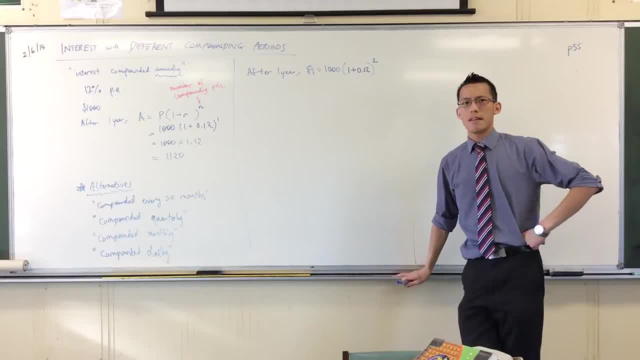 This is not actually how much interest you get Any takers. Anyone see what's wrong? Well, yeah, so it's times two. well, to the power of two, rather right, But you're getting the same amount of interest, right. 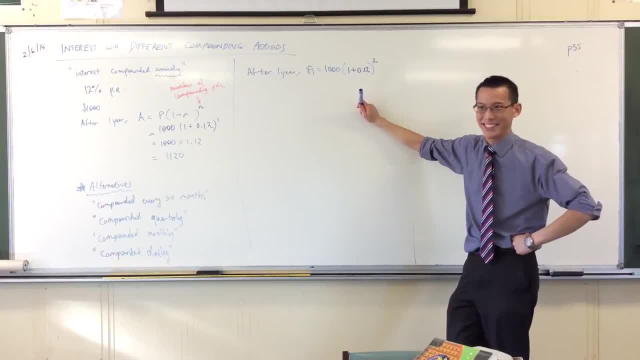 That's a really good deal. That's an incredible deal. It's a rip off for the bank actually. okay, They're paying you the same amount of interest, It's the same amount of interest, but you have to wait only half as long. 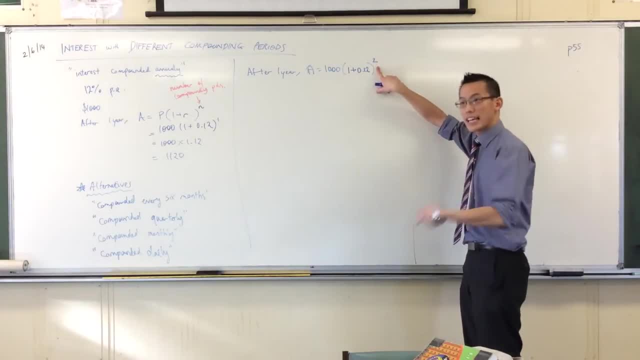 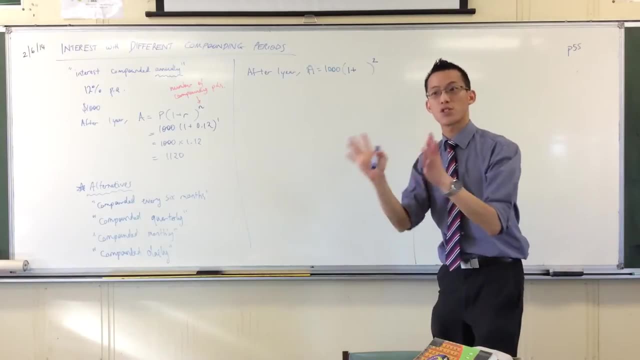 That's not the way they do it. okay, If they're going to recalculate twice as often, they're going to change this number in here. If they do give you interest twice as often, they're only going to give you half as much. 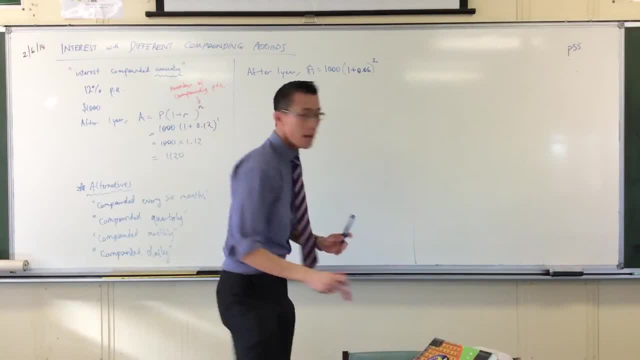 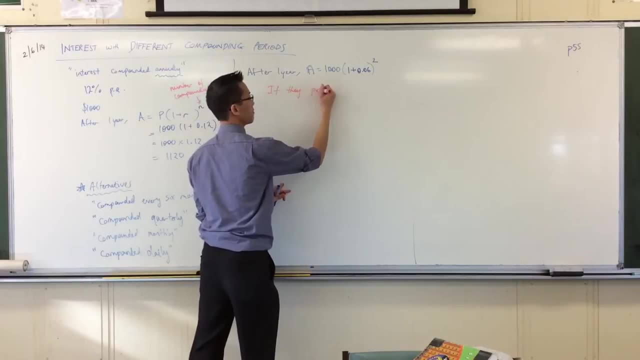 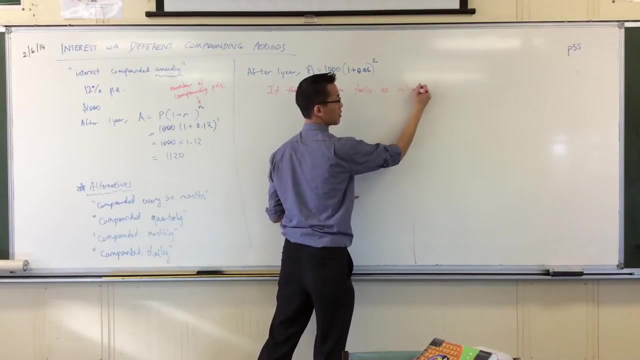 Let me say that That's a really important idea. I'm going to write it underneath for you. okay, If they compound or pay you twice as often, Okay, So instead of once a year, they do it twice a year. Sorry, what's that? 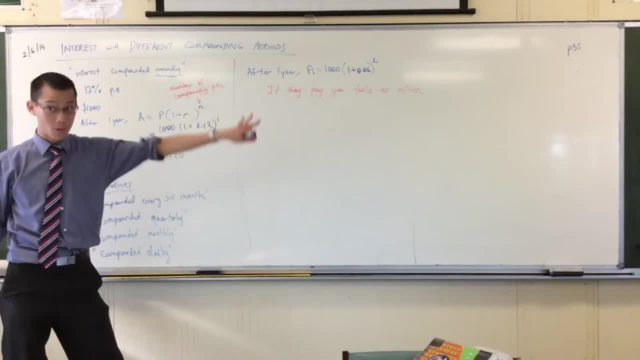 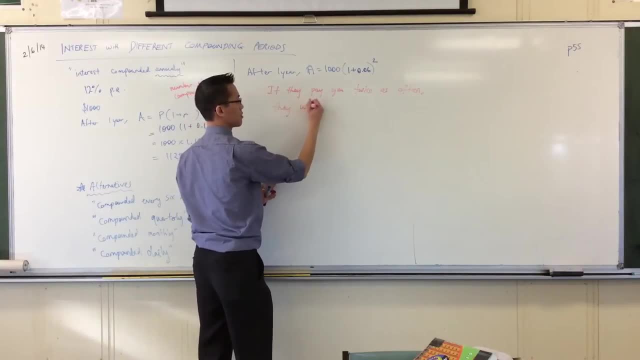 What did they calculate to be more or less the same? Well, we'll see in a second. It will be close, but it won't be the same. If they pay you twice as often, they will pay you half as much. I really need a new red pen. 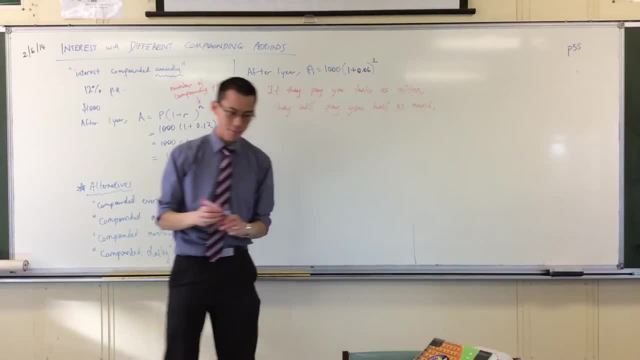 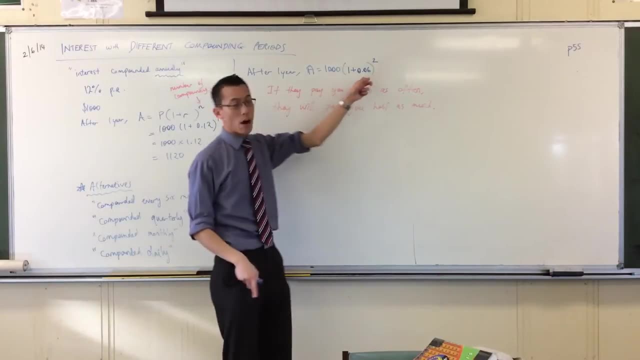 Okay. So can you see what's happened here? 12%: They're going to give you interest over a whole year, but if you say I want it more frequently, they'll say: fine, but we won't pay you as much each time. 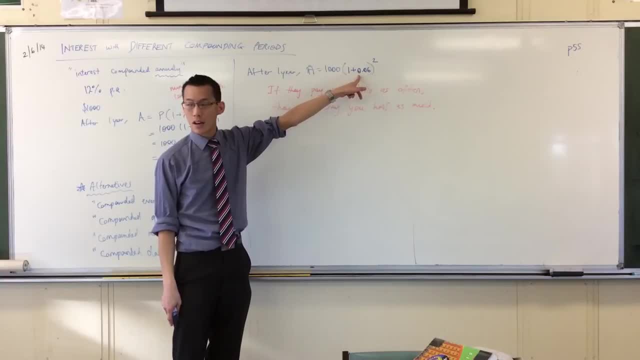 If you want it twice as often, you get half as much. okay, What if we went the next step down, compounded quarterly? okay, It's going to be well, I'll have my 1,000 at the front, right? 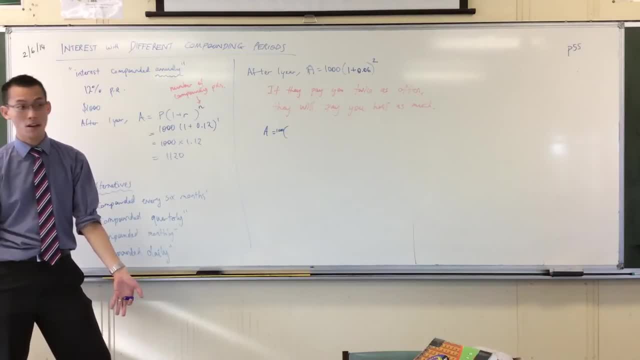 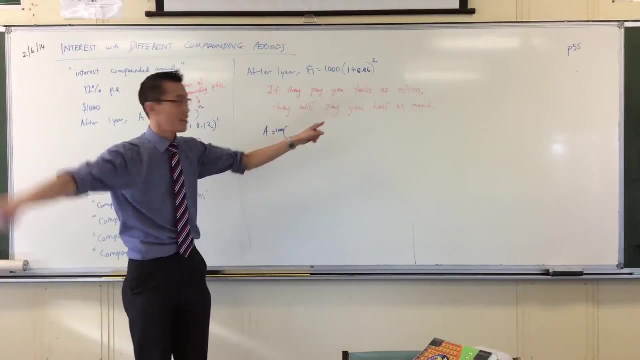 How many quarters are there in a year? They're quarters, right, So it should be four. But they'll say: if you want to get paid, If you want to get paid four times as often, then they'll only pay you a quarter of that. 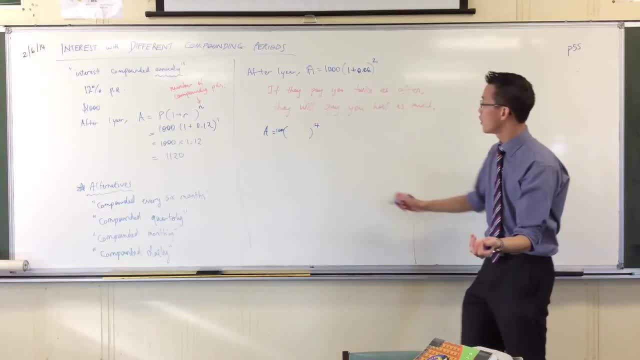 which is a quarter of 12%, is 3%. okay, So I'm going to have 1 plus 0.03,. okay, So can you see this number's getting bigger and this number's getting smaller. This number's getting bigger, this number's getting smaller. 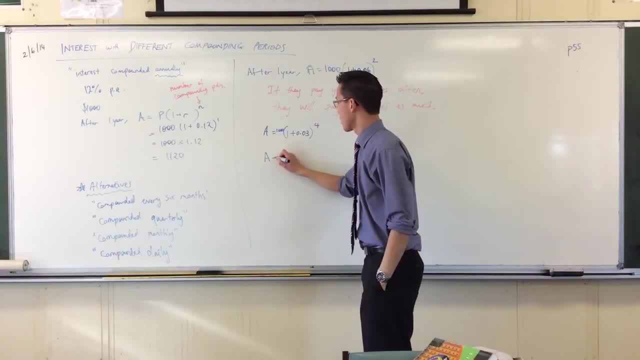 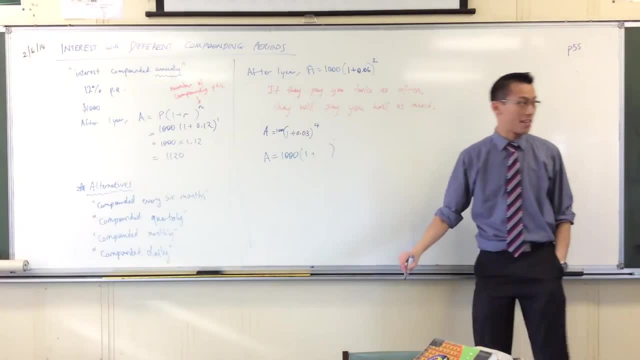 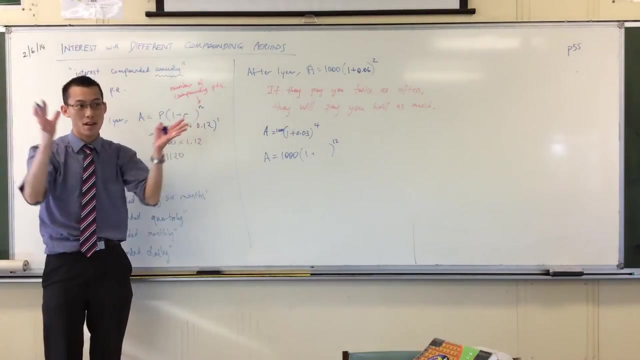 Let's go another step. What if it was monthly? What would you get? You're going to have 1,000 at the front, right? Okay, Now how many months are there in a year? There are 12.. So, being that they're paying you 12 times as often they're going to pay you 12 times. 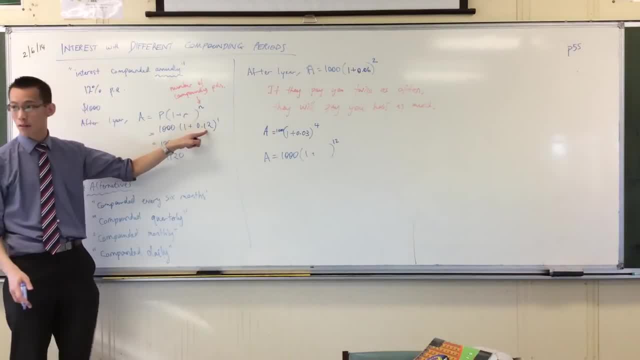 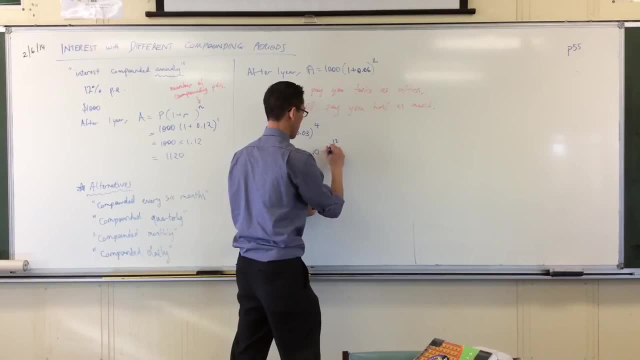 less the amount Now. it was 0.12 before right, or 12%. So how much are they going to pay you each month? It'll be 1%- 0.01.. I have a quick question for you. 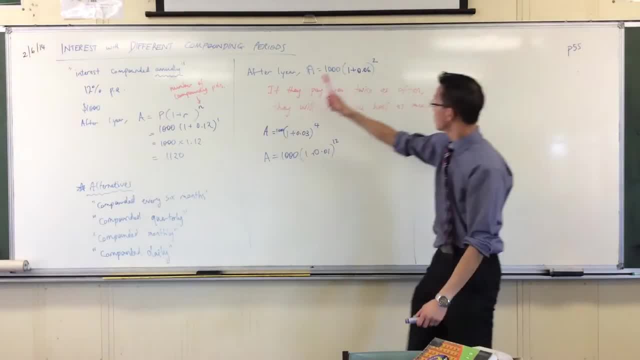 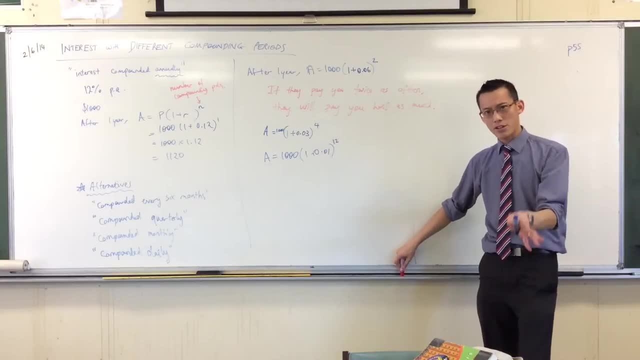 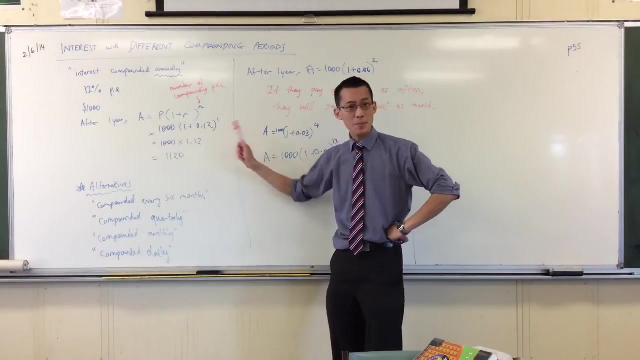 I've got- let's see, Sorry, One, two, three, four amounts on the board. Don't say it out loud, Just think about it in your own head. Which do you think would be the best deal, right? Is it better to get less payments but one big hit, right, or a bunch of smaller payments? 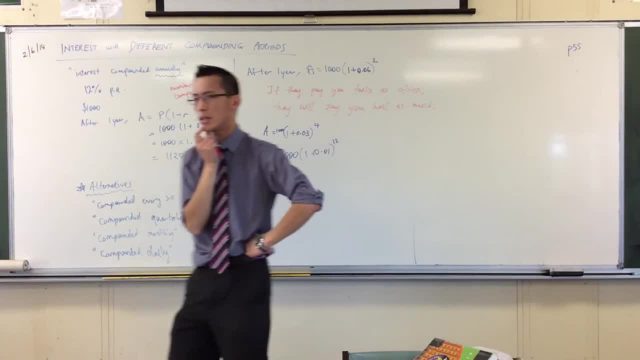 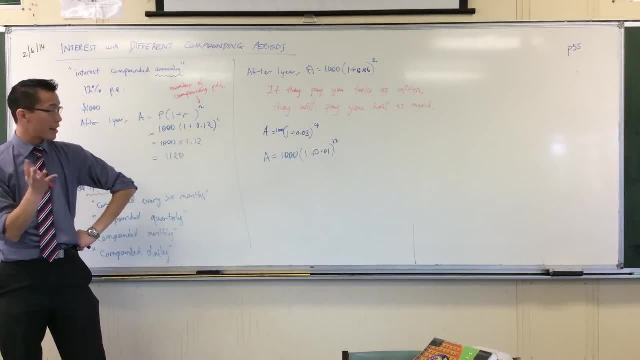 but more of them. I wonder which one we're making. Yeah, Yeah, We don't need to guess, because we have calculators that can do this for us. right? We've already done it here. Compound it annually, There's our amount. 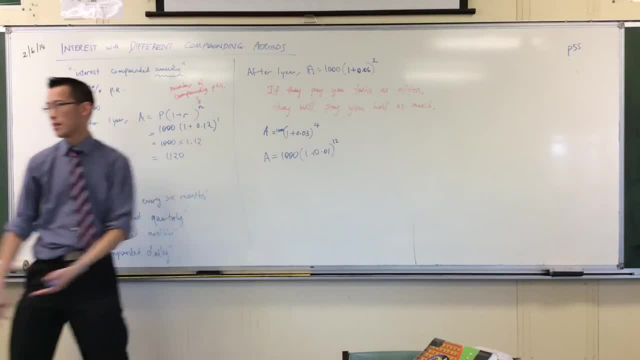 Okay, Now I've got three more here, So maybe what I'll do is: here we go, you guys, you seven. okay, can I get you guys to work out what this number is? Can you get your calculators out? 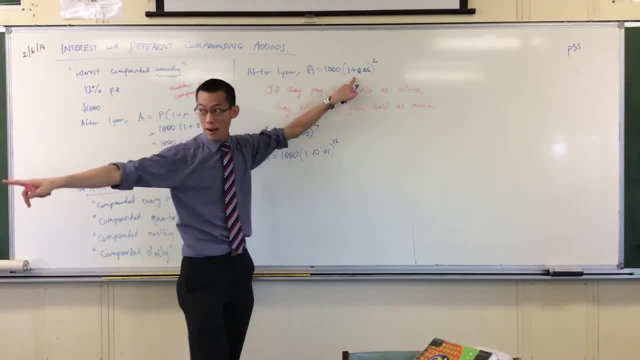 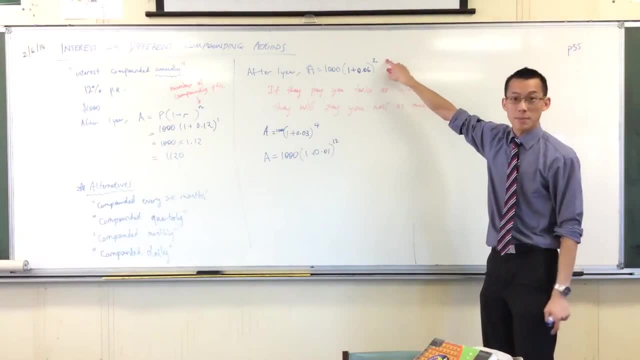 Get your calculators out and calculate this number. Wait for it. if you've already got it, You guys in here, actually the whole middle, the whole middle. can you guys work out this one? So this is six monthly, right? This is quarterly. 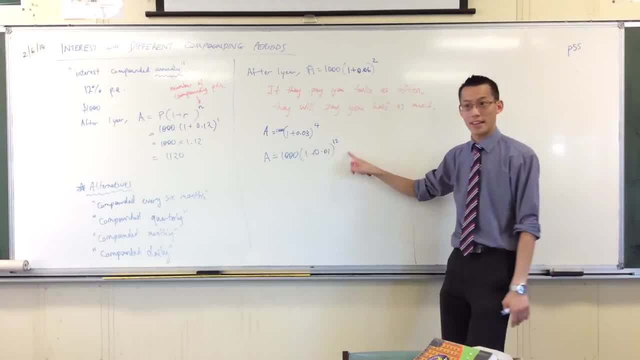 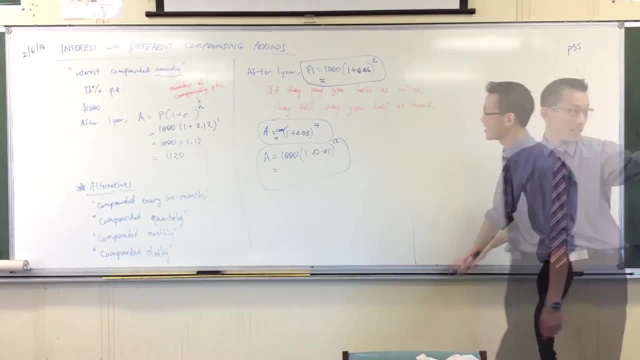 And can I get you guys on the right-hand side of the room to work out monthly? Okay, Well, they're going to be all different answers. They are going to be all different answers. I hope they're going to be all different. 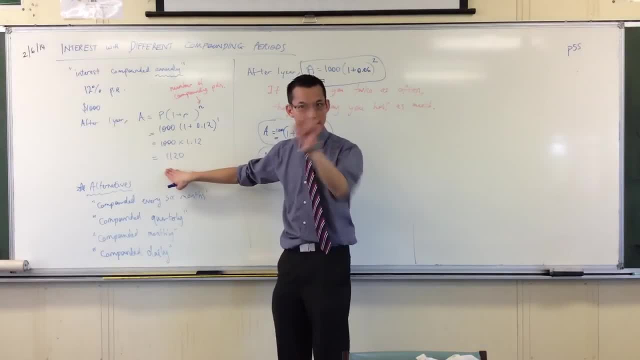 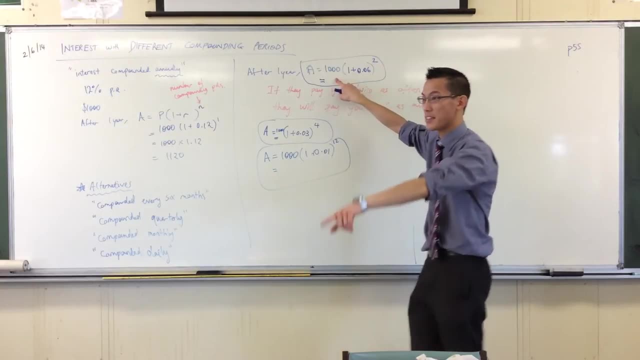 All right, Let's start with: we've done compounding annually. So there you go, There's a number. All right, Let's see. Jared, can you give me compounding twice a year? What do we get? 1.11.. 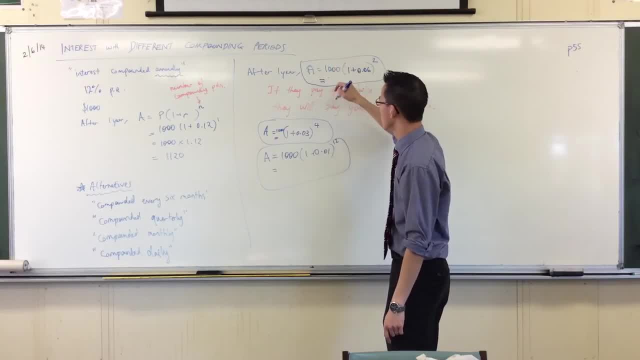 Hold on 1.12.. Wait, You said it's a year's cent. Yeah, So it should be 1,000 and something right. What I've got here is 1.1236.. I think you mean 1,000.. 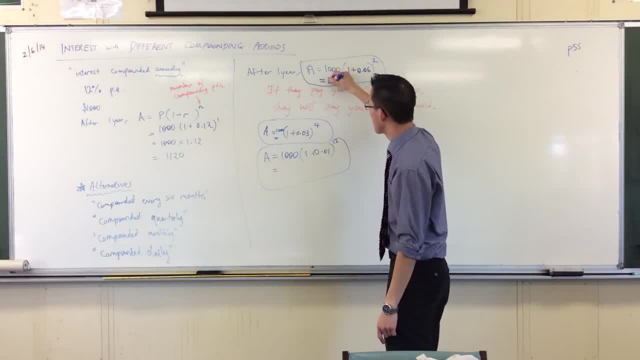 Did you multiply by 1,000?? I put that in, I just didn't put the 1,000 in. Oh okay, All right, So can you multiply by 1,000? So we'll get 1,100 and. 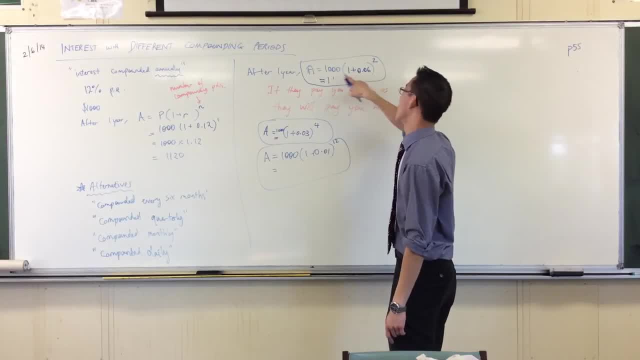 Yeah, 1,123.6.. Six and zero, Yeah, Okay. So hold on. $3.60. better than there. Same amount of time, but more frequent, Okay, $3.60.. $3.60. $3.60.. 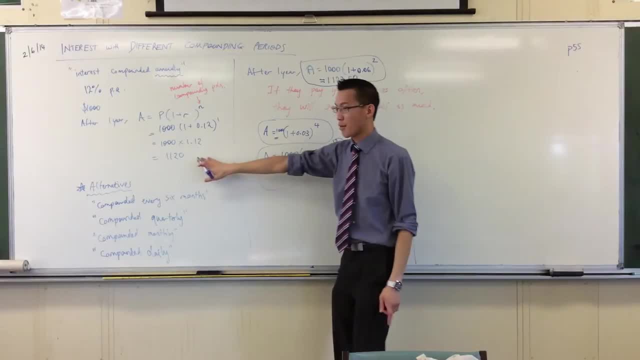 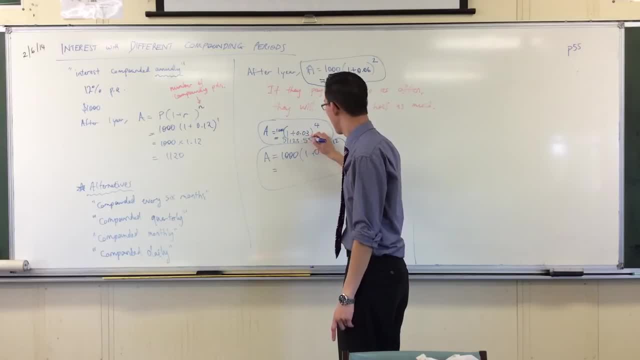 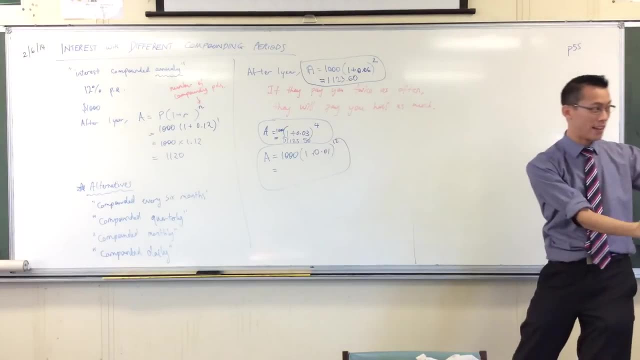 $1,125.50?? Yeah, $1,125.50.. Okay, Better again. Same amount of time, smaller amounts of interest, but more of them, Okay. Final answer: Yeah, Luke, I've got 1,126.. 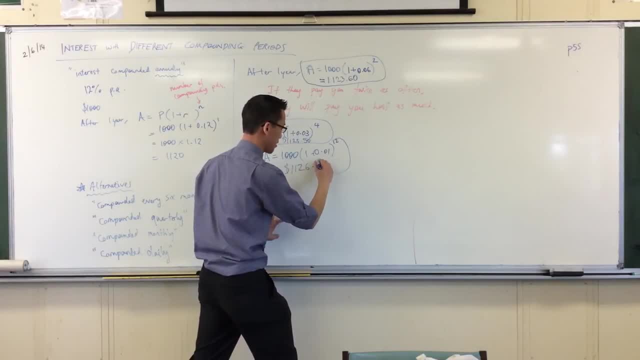 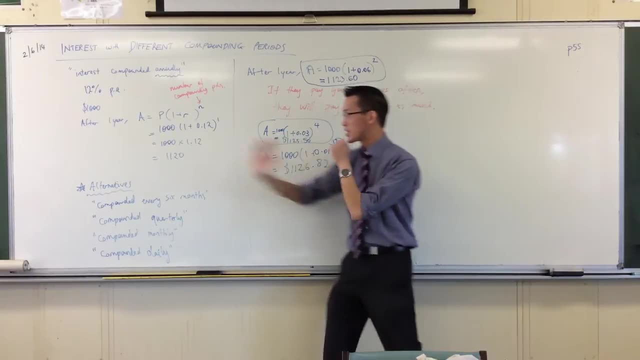 1,126.. Eight, Eight And nothing after that. Three, Two, Two, All right. So let's have a look. Let's compare our numbers, shall we? Okay, We started with this: $1,120.. Okay. 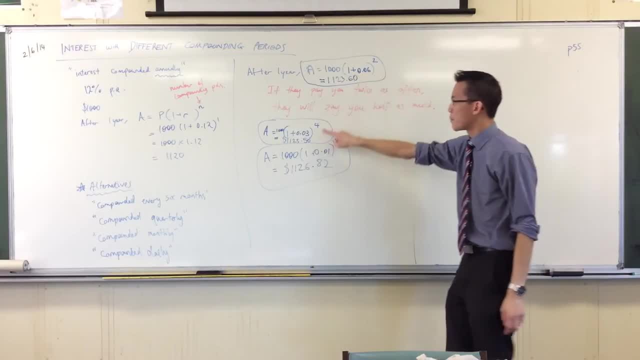 Then we got a bit extra here, and we got a bit extra here and a very little bit of extra there. Right, In fact, you can see the further I go from here to here, I gained like $3.50.. 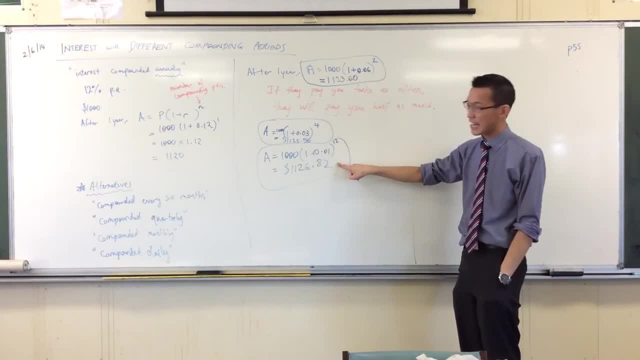 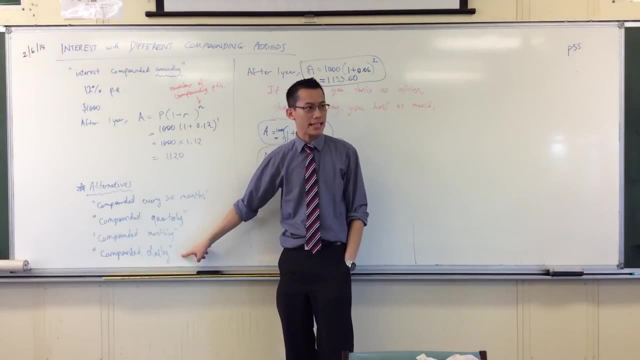 From here to here, I only gained like $2.. From here to here, I only gained a bit over $1.. I'm actually slowing down, Right. This is interesting. I left off one more compounding daily. We haven't done that. 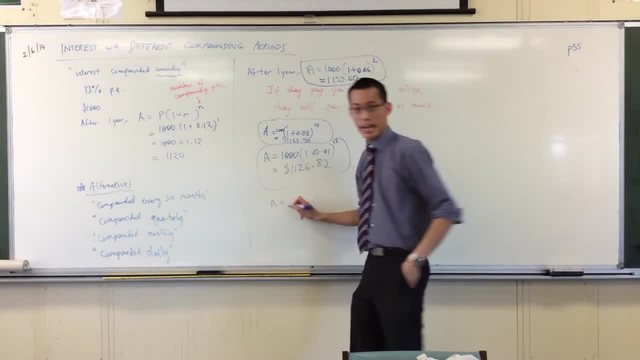 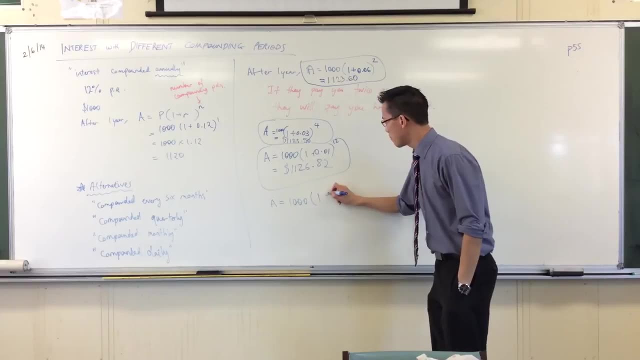 Let's do that together. Okay, I'm going to say amount. Okay, And this time I want you all to write this down with me, because it's the trickiest one. The principle is still the same. Okay, It's going to be 1 plus. Now, what am I going to put in here? 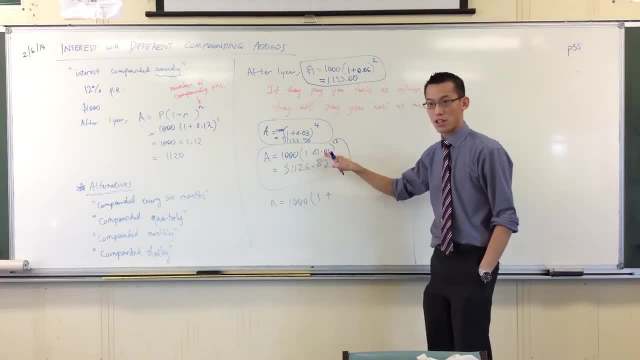 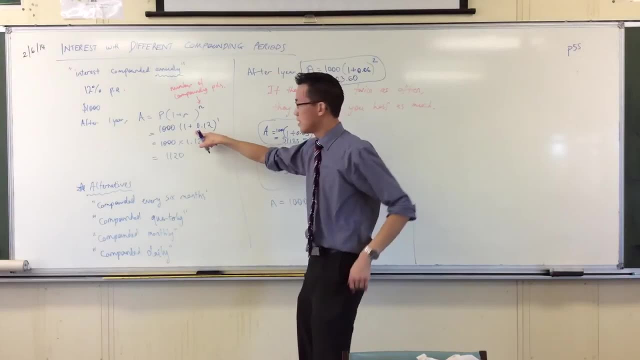 It was nice easy numbers here, right: .06, .03, .01.. What's it going to be Well, 0.06.. Let me put this to you, okay, This is 0.12 per annum. 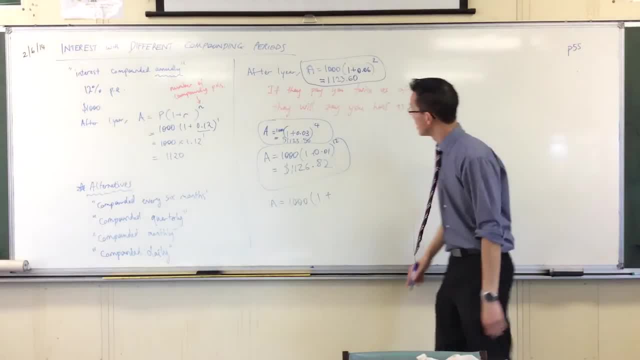 Right? How many annums are there? There's one. There's 0.06. here It's actually 0.06.. It's actually 0.12 divided by 2.. Why do we divide by 2? Because it's half a year. 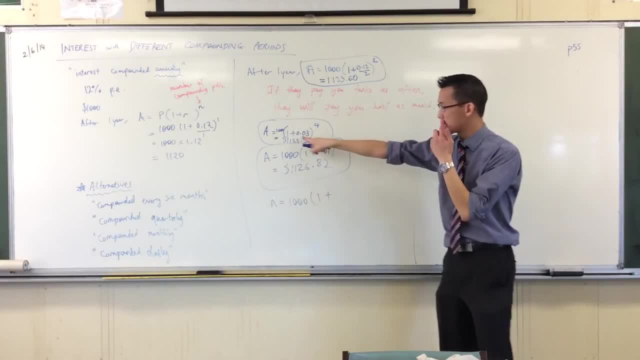 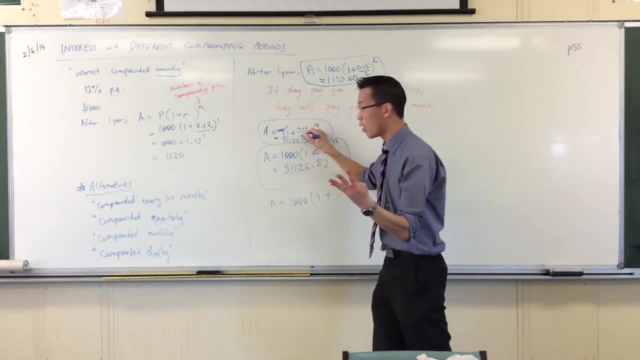 It happened twice a year, didn't it Right? Six months is half a year. What's this number? .03?? It's actually 0.12 divided by what Four? Four, because it was quarterly, Quarterly. Can you see this number and this number? 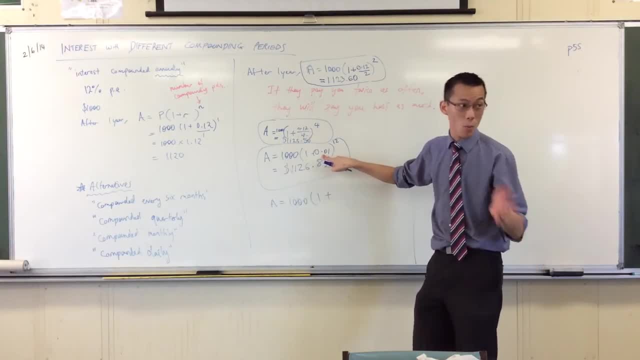 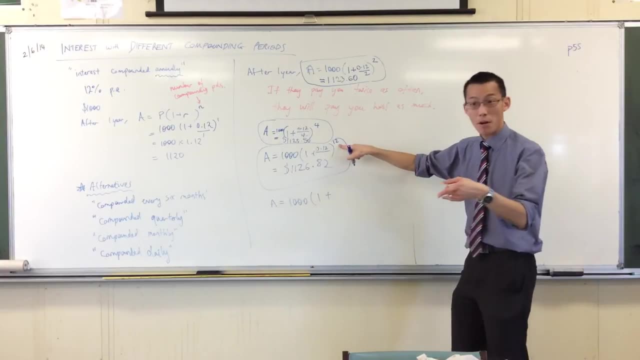 It matches. Can you see that? And here, of course, this 0.01, where did I get it from? Where I got it from was 0.11.. Okay, 0.12 divided by 12.. This number up here. 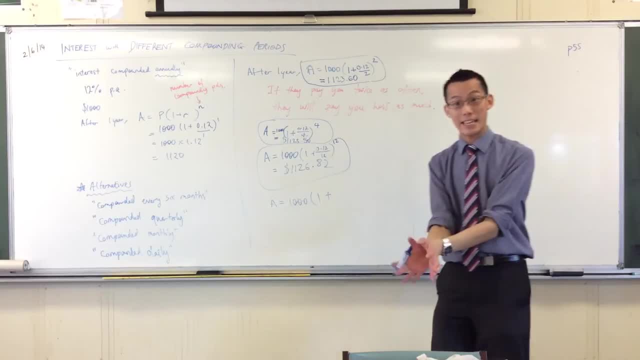 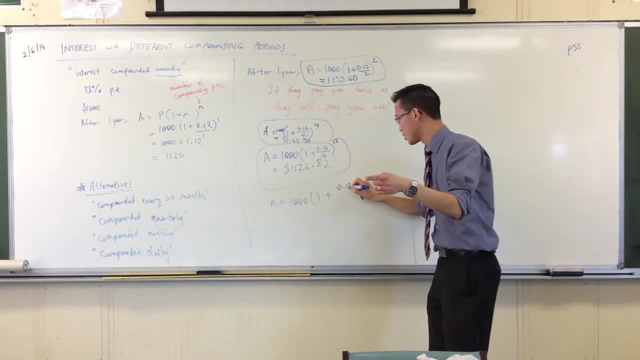 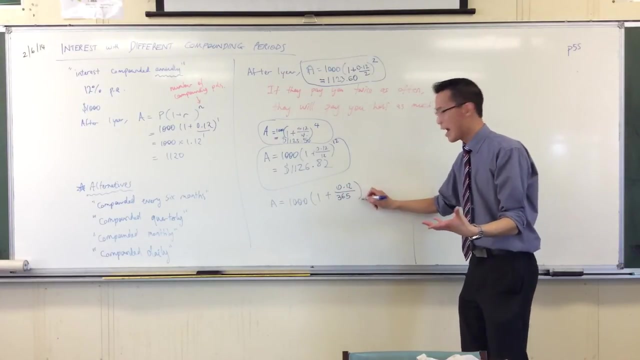 Right Now. therefore, if I want a year in days, not in six-month lots or three-month lots or one-month lots- 365.. Yeah, It's going to be 0.12.. That's your rate, Yeah, But I divide it by 365, the number of days there are, and then I have to raise it to. 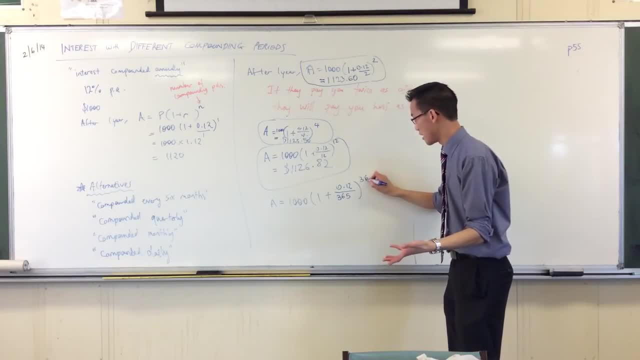 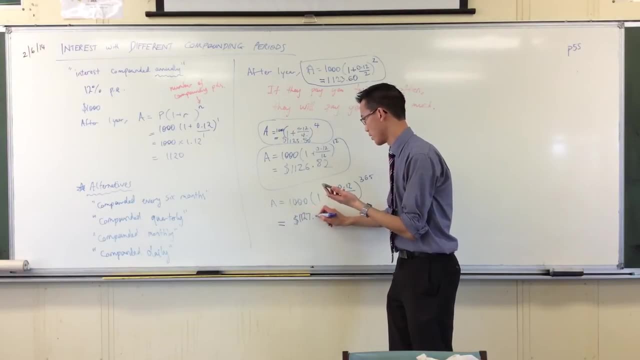 a power of how many days there are in a year, which is still 365.. Okay, Let's get the number One. one, two, seven. Yeah, That's what I got. Oops, Sorry, Left off a one. 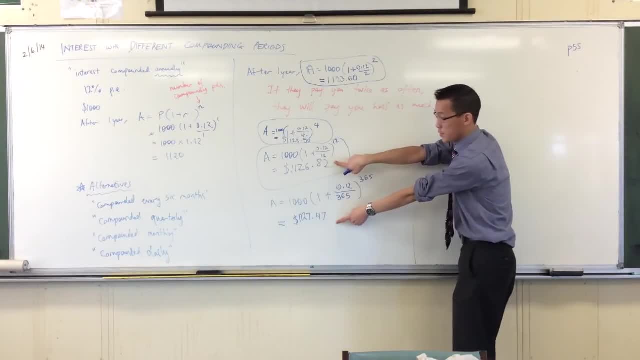 Okay, Look at this. Compare these two numbers. What's the difference between them? It's higher, It is higher, Though not much is it? How much did we gain? We didn't even gain a full dollar. We didn't even gain a full dollar. 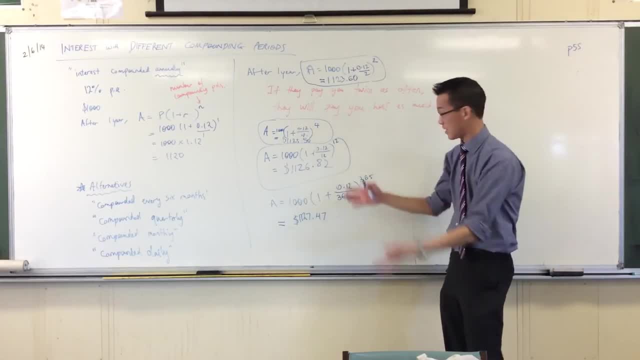 We gained like 60 cents, 65 cents. Okay, So you can see I do get more. So, in answer to our first question, which is a better deal? is it better to get one big chunk of interest all at once or is it better to get one big chunk of interest all? 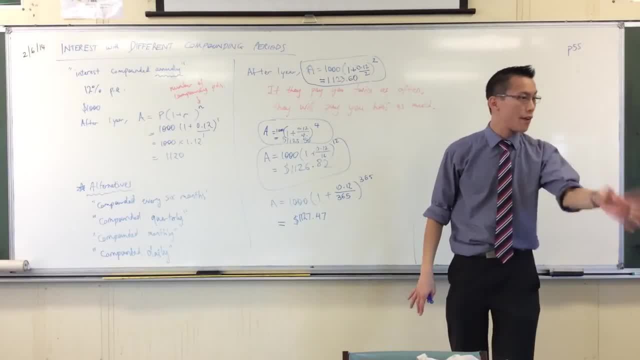 at once, or is it better to get one big chunk of interest all at once? or is it better to get little bits of chunks of interest but lots of them? The answer is: get small chunks of interest and lots of them. That's a better deal. 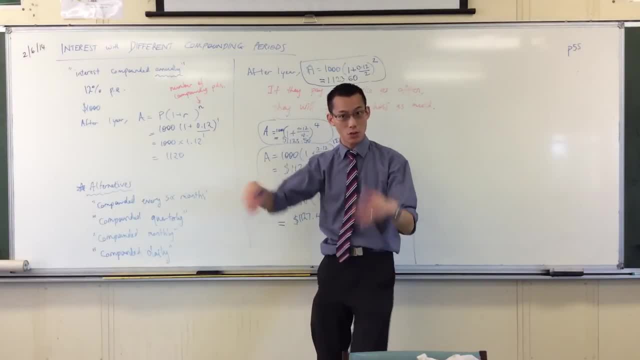 So all the time? Yeah, What about lots of chunks of big interest? If you have a bank account that will give you lots of chunks of big interest, then ask them about their fees, just in case they're charging you some crazy amount. 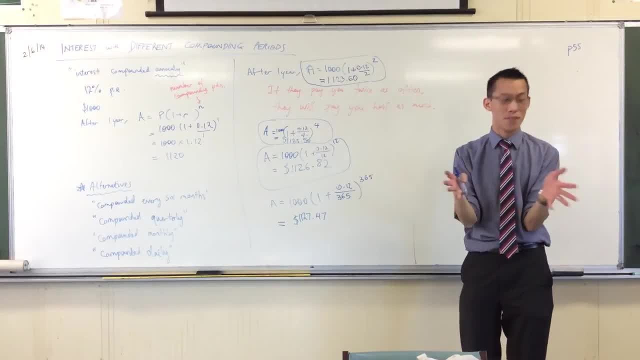 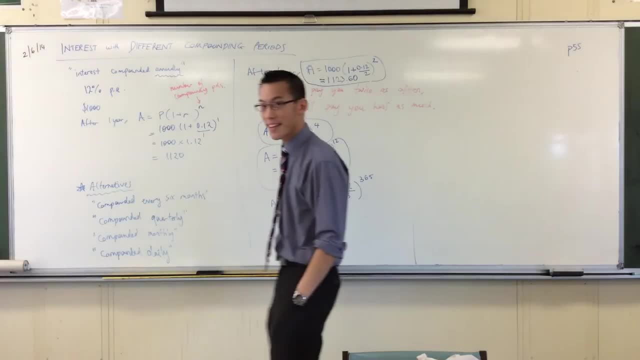 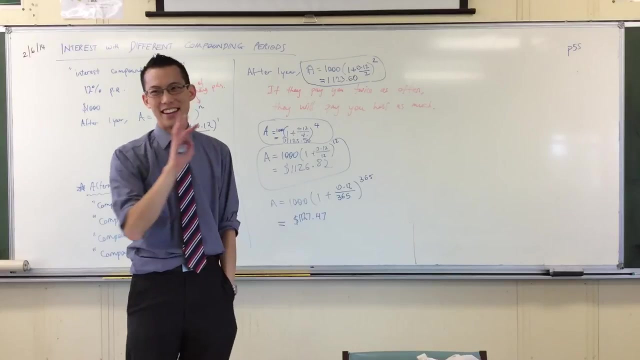 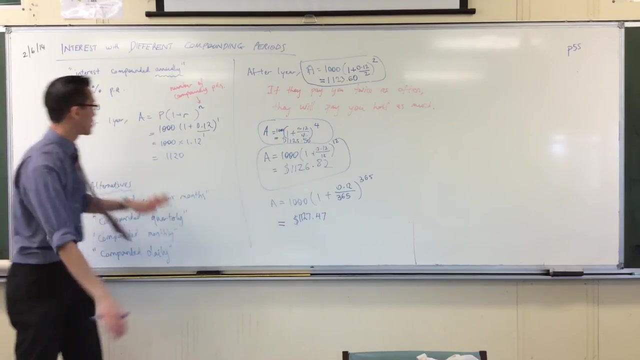 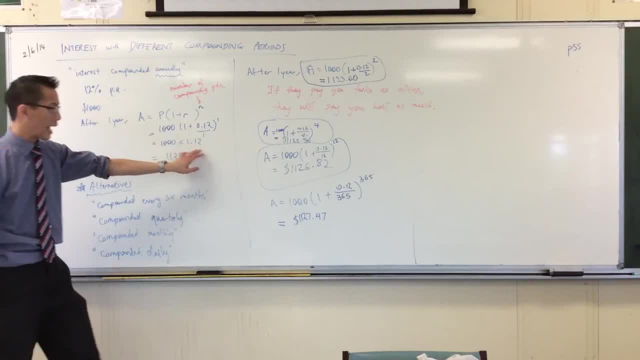 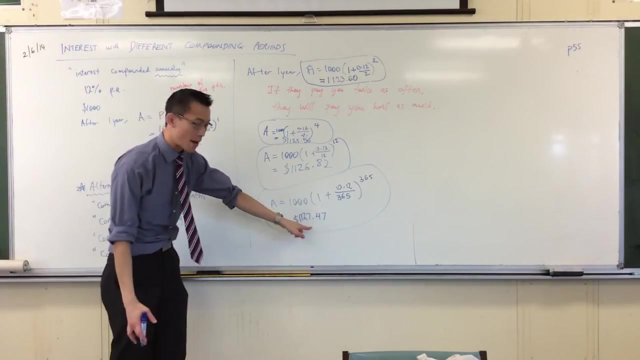 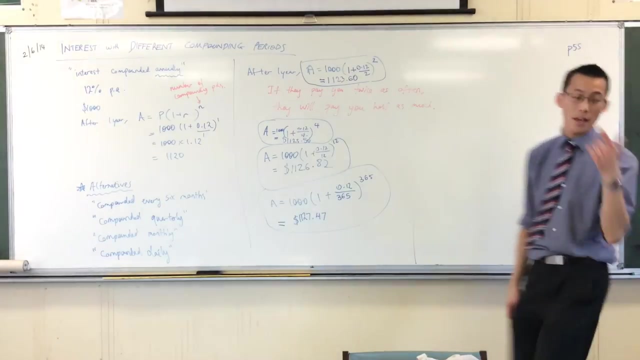 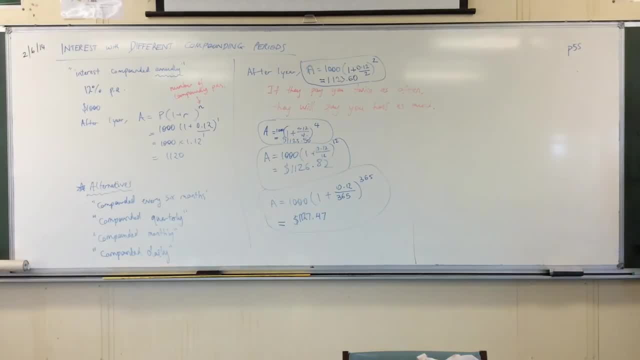 Just look at this middle one under question 8, and you've got a whole bunch of different options. Stop doing that, That's better. Okay, Now have a look at these different options. This exercise has that big table just before it. 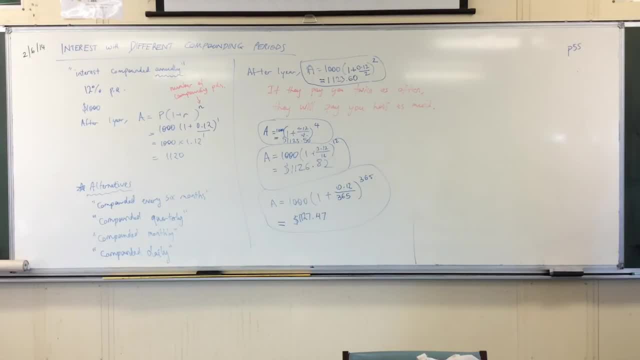 This one, This one. Remember that? Do you remember it from last week? Okay, Now, the way we read it was: you look for an interest rate across the top. That is page 59, and this table is page 57.. 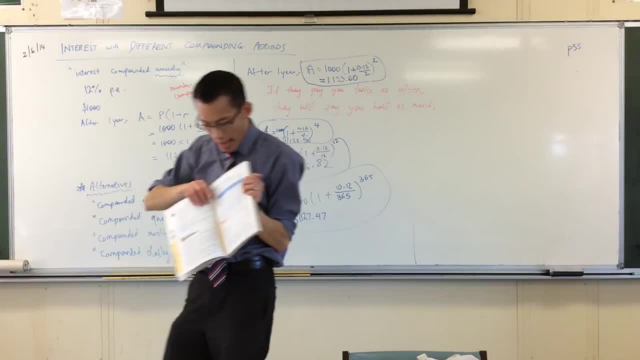 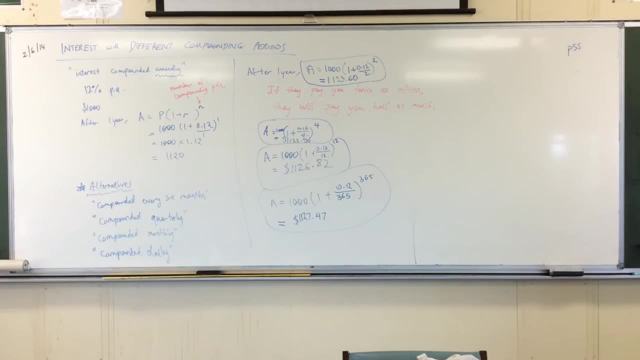 Okay, So we read across and we said: look an interest rate up here. And then we looked for a time down the left-hand column and then you matched up whichever cell you were supposed to be in. Okay, Now have a look at this, for instance: 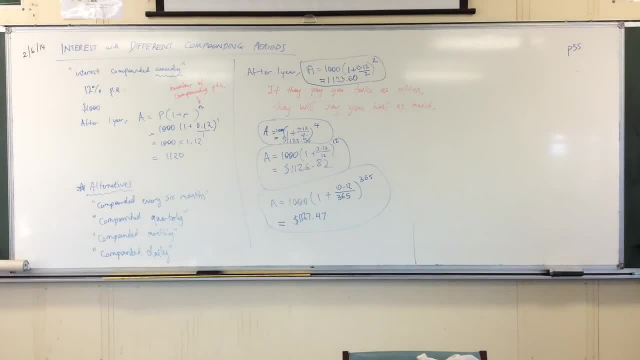 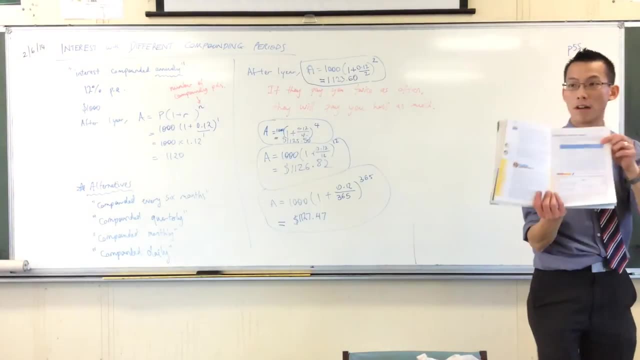 See this one in here, right, 10% for four years. 10% for four years. Now, if that's all you knew. you would go across to the 10% column right right along the end, and then you would go down to which row. 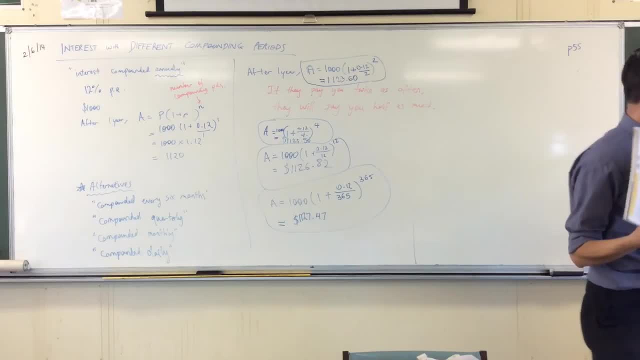 Which row would you go to? Row number four: right 10%, for four years, 10%, And you get another Number: there it is 1.464.. Okay, Ah, but then they tell you something else.